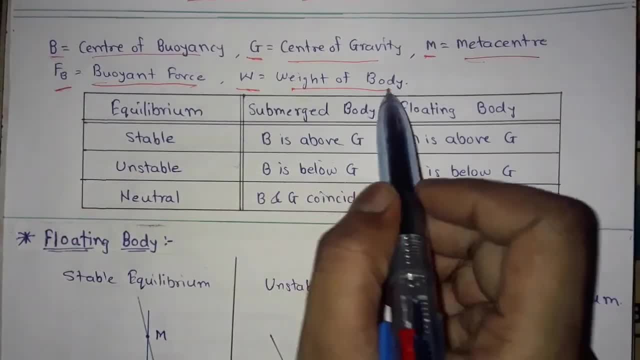 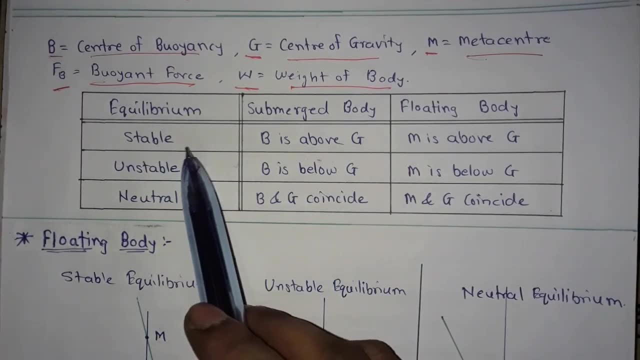 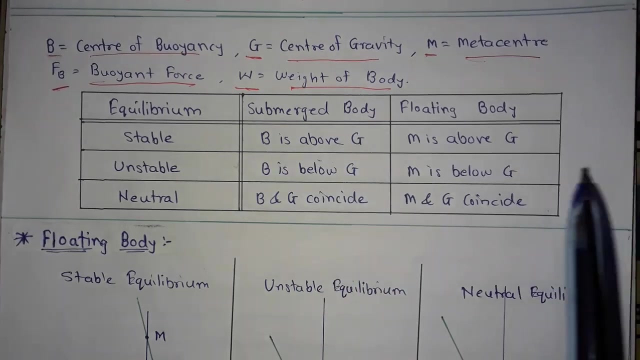 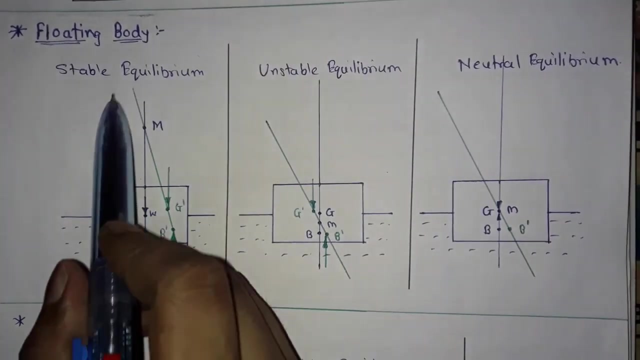 buoyant force, W is for weight of the body. and this is the tabular representation of various cases of equilibrium: stable equilibrium, unstable equilibrium and neutral equilibrium for submerged body and floating body. so, friends, let's start with the floating body. first is stable equilibrium in stable equilibrium. friends, in case of floating, 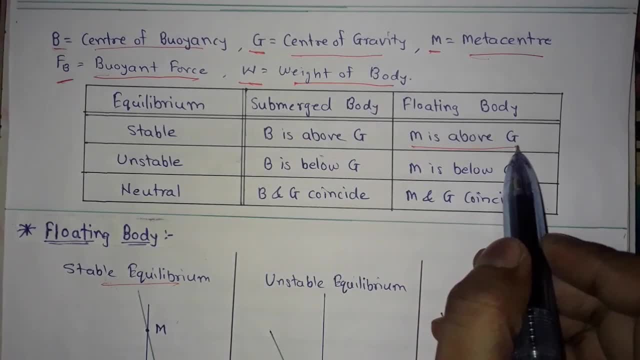 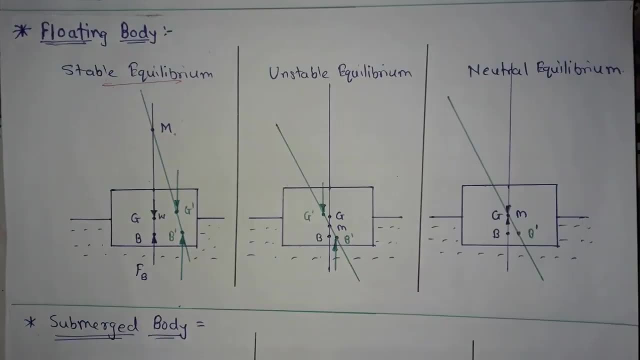 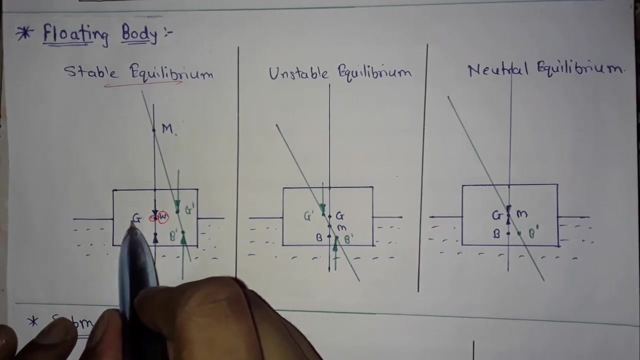 body, M is above G, that is, metacenter is above G. here, friends see, M that is metacenter is above G. in this case, friends, weight of the body, that is, W, acts below at the center of gravity. here, and this is the point B, where force of buoyancy or buoyant force acts, this is the center of. 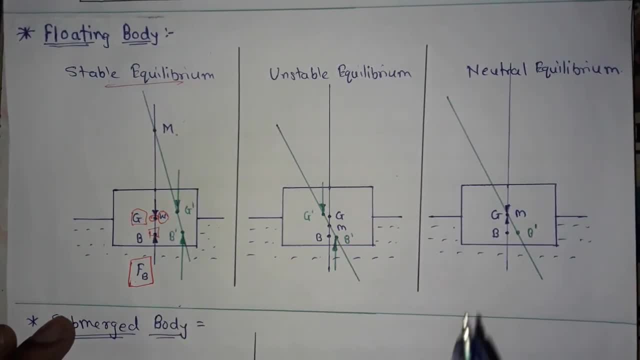 buoyancy. friends, if you want to know more about buoyancy then please watch my video related to buoyancy and Archimedes principle. the link of this video I have given in the description section of this video. now, friends question is how this meta center we have? 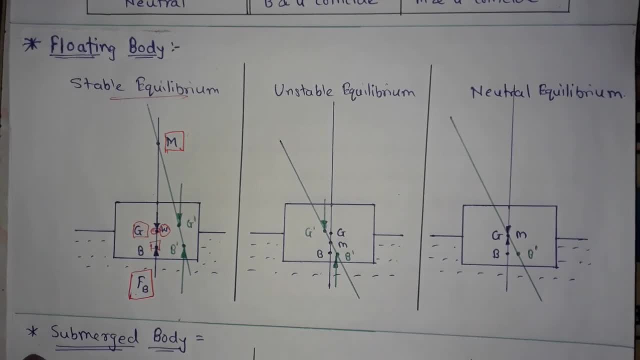 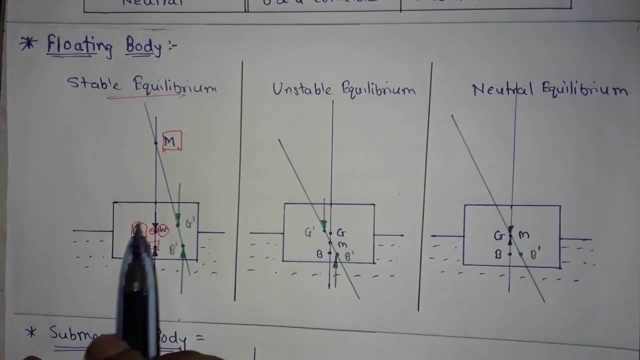 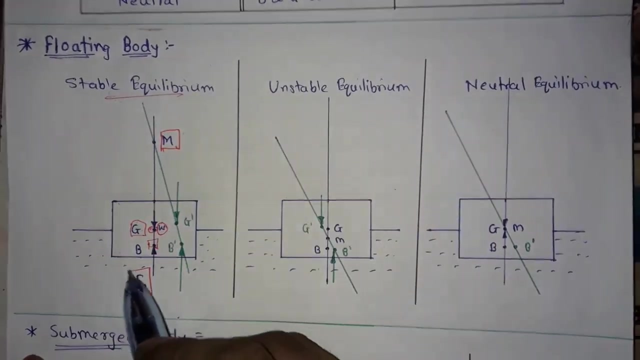 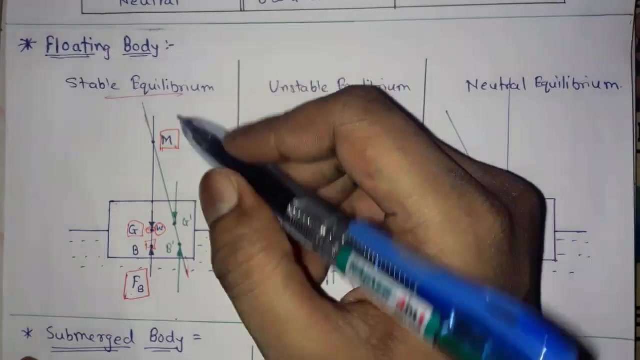 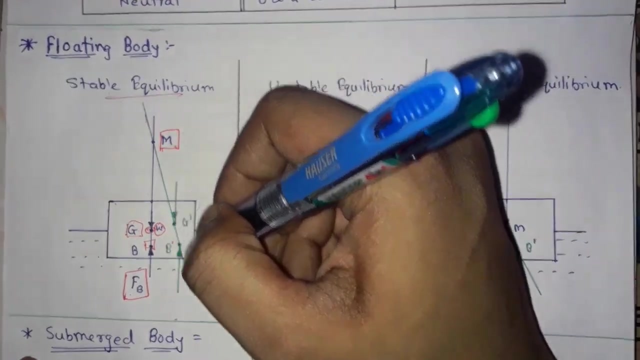 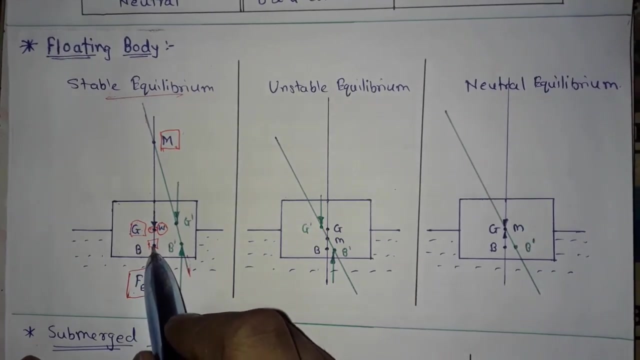 got. suppose, friends, this is the original position of this floating body and if suppose, friends, we displace this body from this position, this is the original axis and this is the displaced axis of this body. so, friends, point G shifted to here on this new displaced body axis, and denoted it as G, dash and B point that. 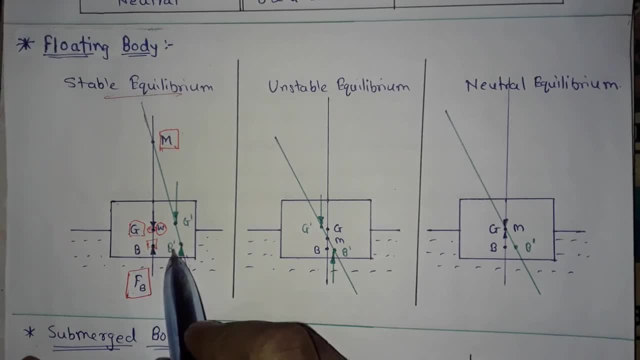 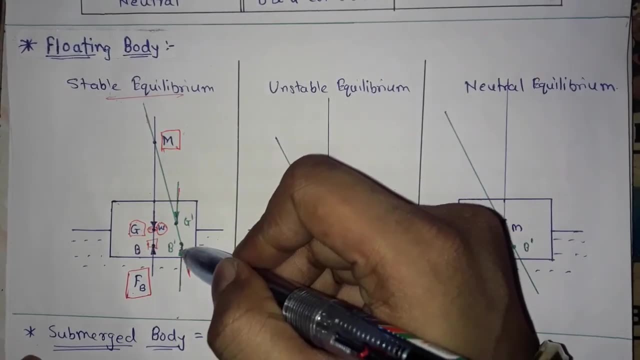 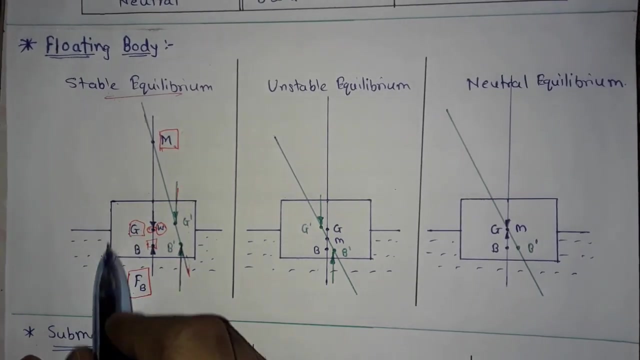 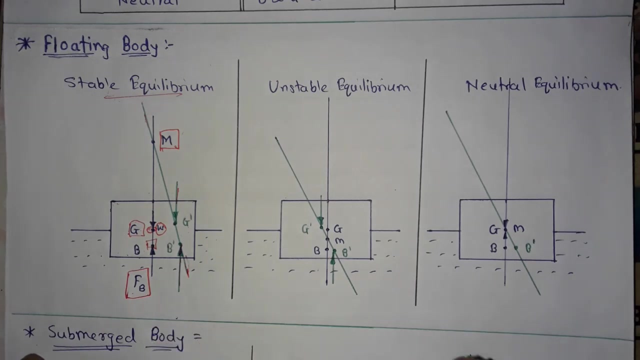 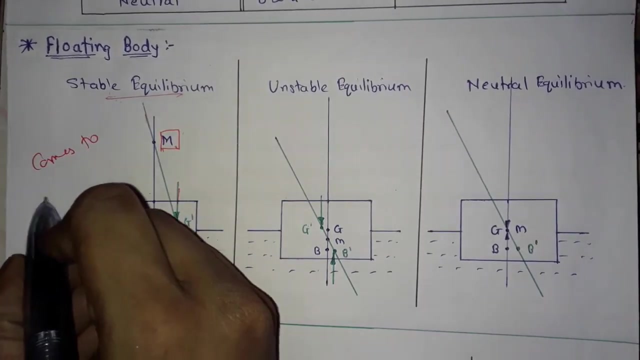 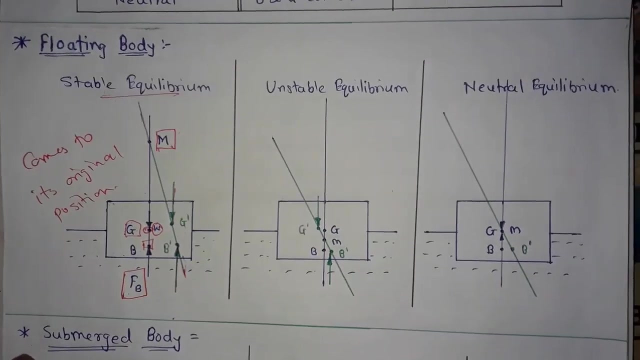 is center of buoyancy. shifted here B dash, friends, in this case due to this couple. this couple, this body again come to its original position, that is this one. this means, friends, whenever we displace a body, floating body, it comes to its original position. comes to its original position. now, friends, let's see the. 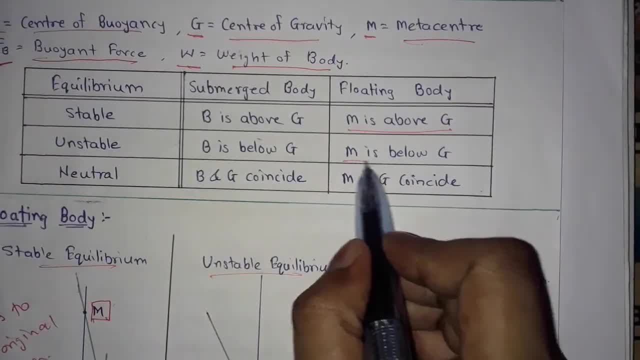 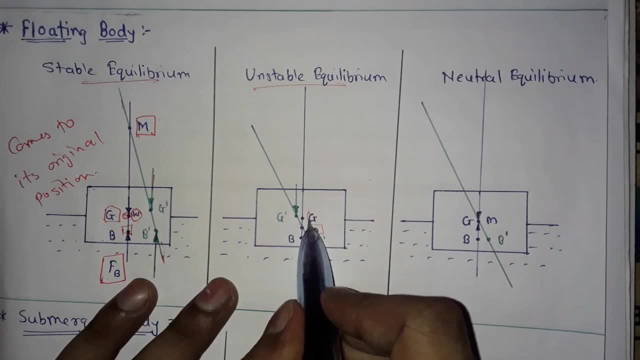 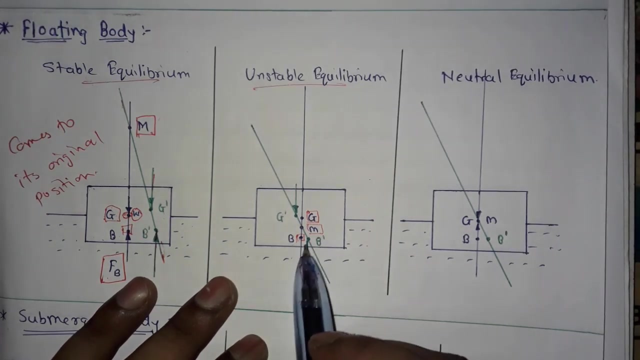 unstable equilibrium, in unstable equilibrium, friends, M is below G, see friends here. M is, that is meta center is below G, center of gravity, and here is the center of buoyancy. now, friends, in this case, also, when we tilt or displace this body from its original position, if there. 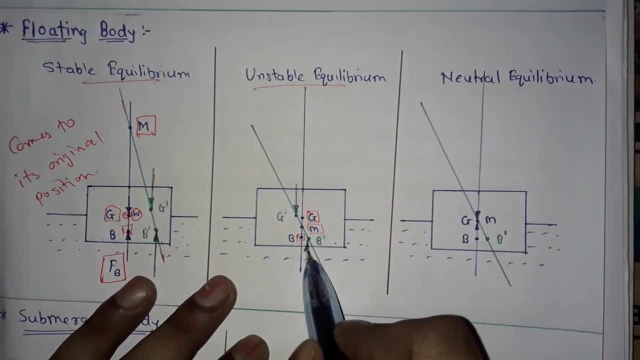 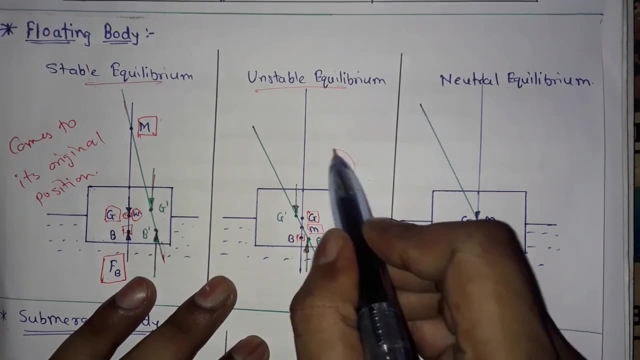 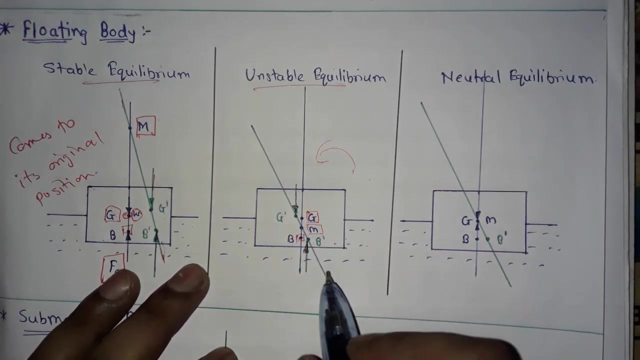 is. there is a couple which acts on this body like this. due to this couple, his body overturns completely. so in this case, if we tilt this body from its original position in unstable equilibrium, friends, when we displace a body from its original position, it over turns. 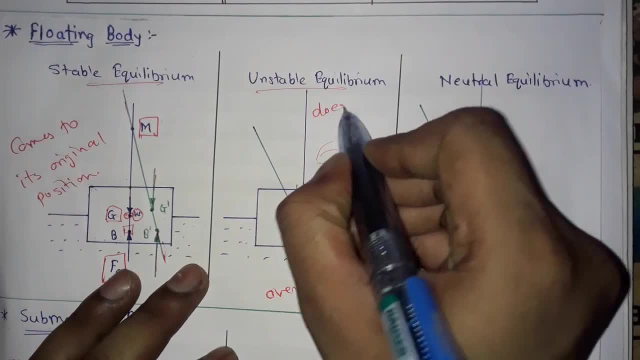 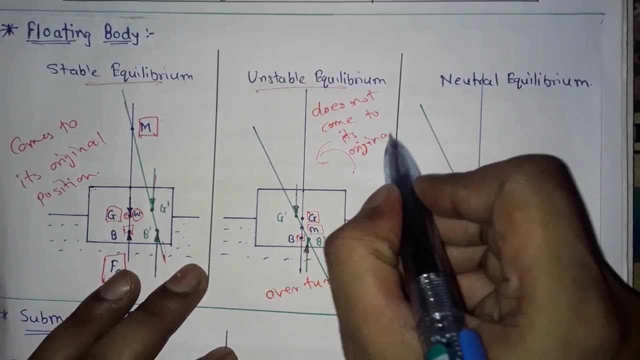 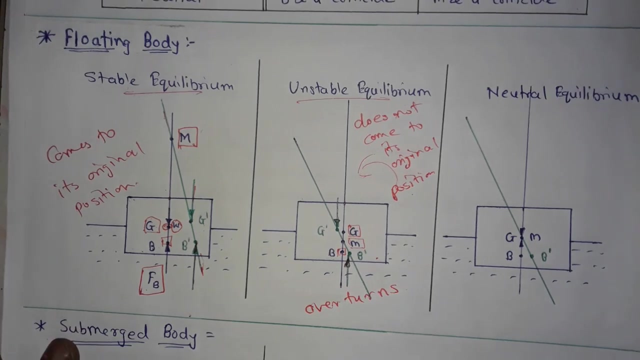 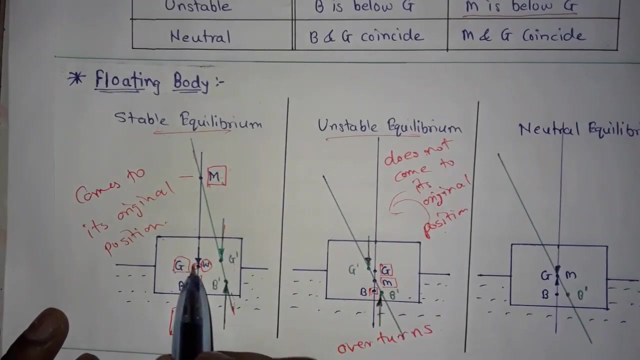 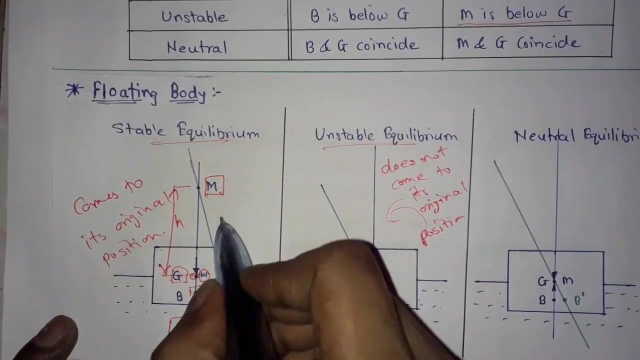 in this case, friends, the body does not come. come to its original position and, friends, one thing is: let's go back to the stable equilibrium. this is metacenter and this is the metacenter height, friend. metacenter height- that is, the distance between the g and m- is called as metacenter height. 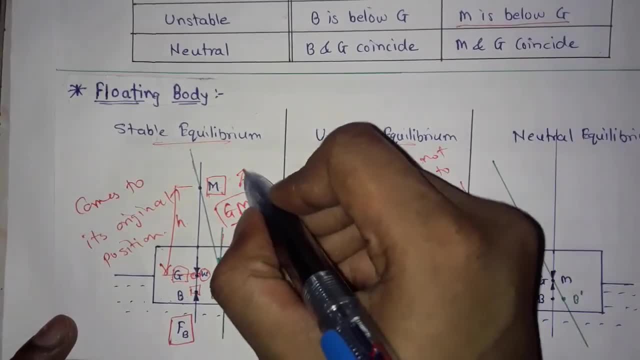 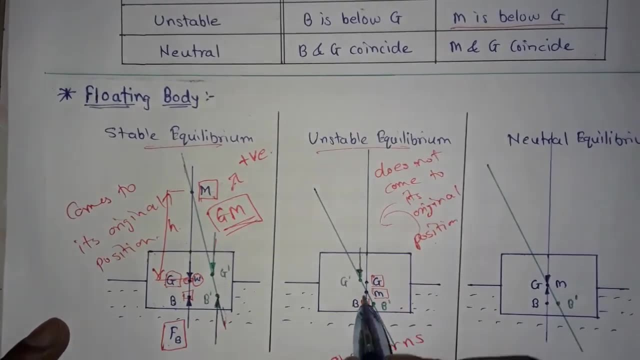 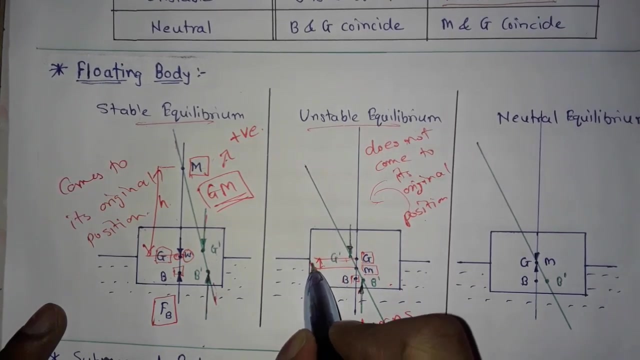 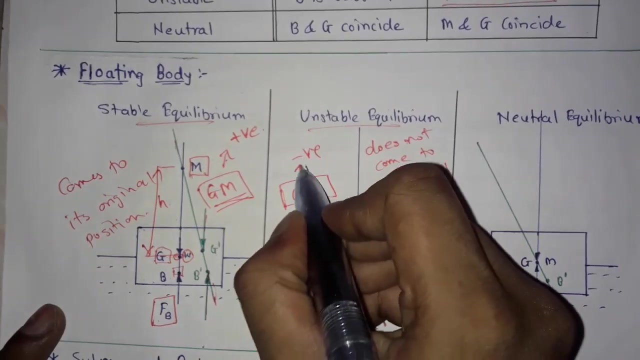 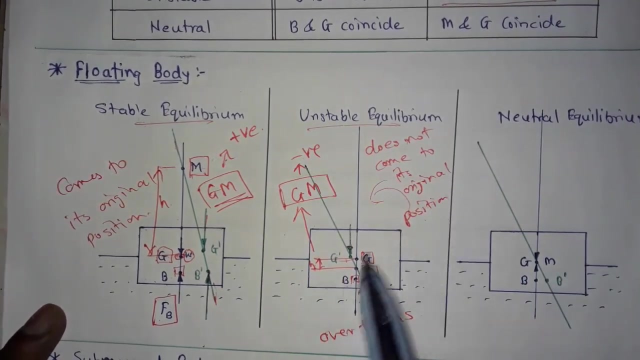 here, friend, in this case, the metacenter height is positive, so it is a stable equilibrium. and here, friends, in this case, as m is below the g, here, friends, this is metacenter height, gm. here, friends, in this case, gm is negative. so in this case, friends, it is unstable equilibrium, that is, body does not commit to its original position. 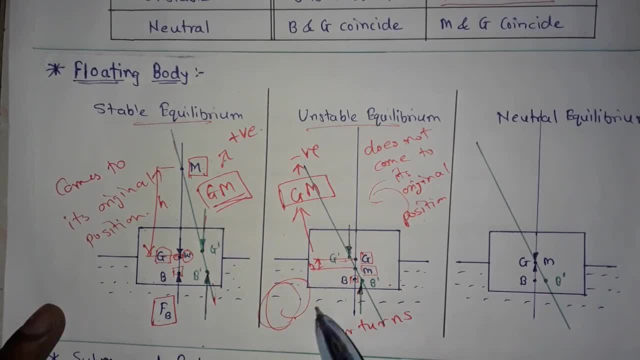 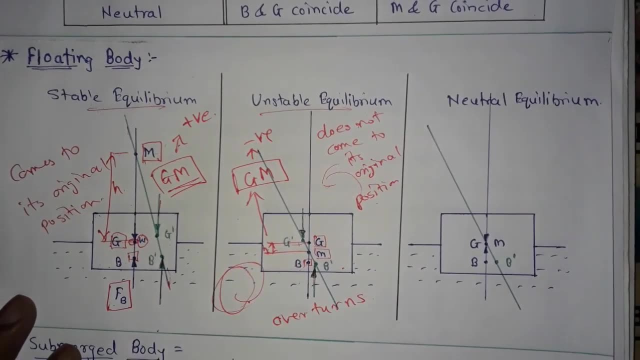 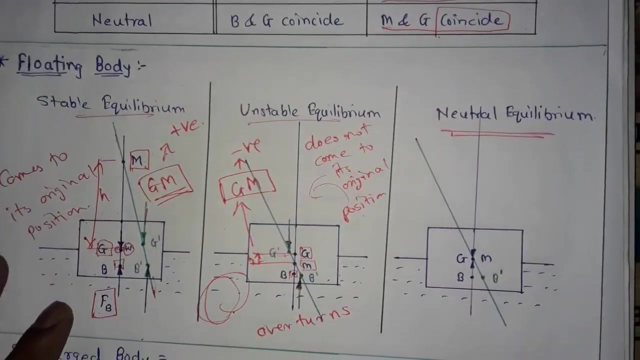 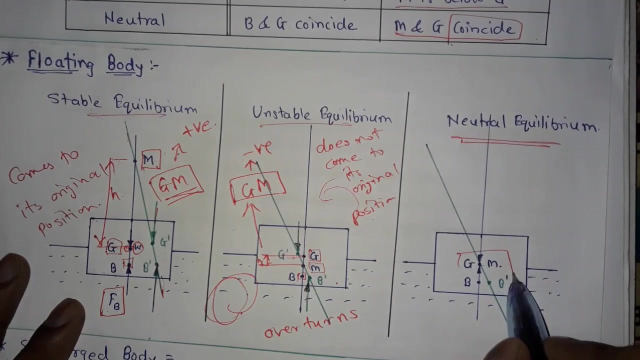 it over, turns like it rotates, like this in. in short, friend, it rotates completely. next is friend, neutral equilibrium. in neutral equilibrium, friends m and g coincide. see, friends, here the metacenter and center of gravity has the same point, that is, it is here and this is the 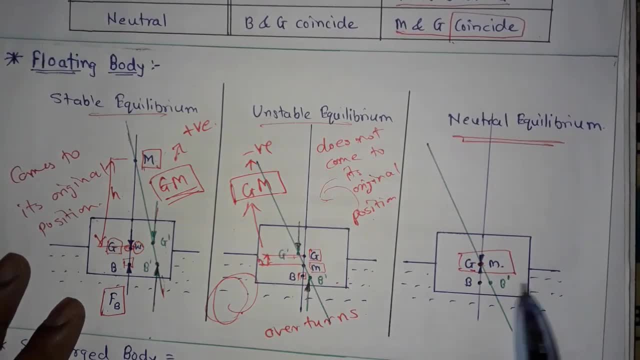 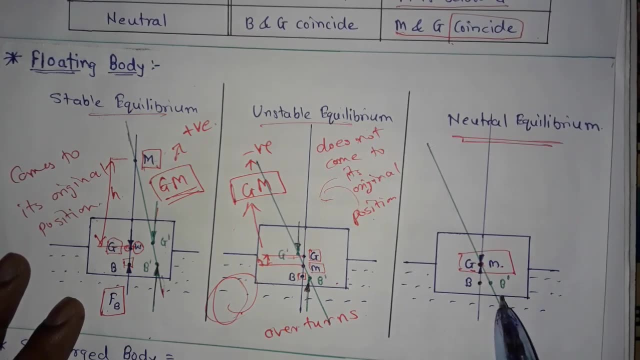 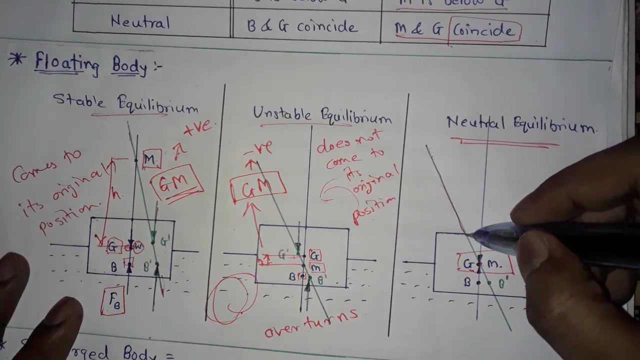 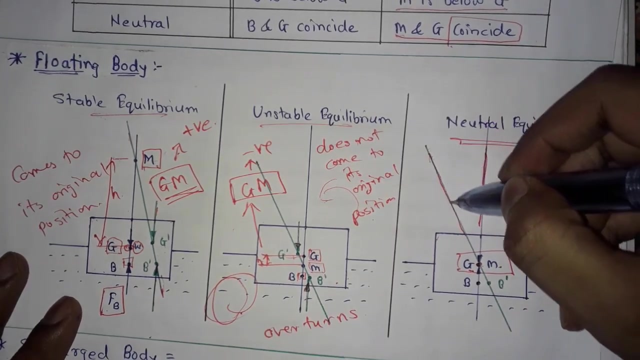 center of buoyancy, where, in this case, friends, when we displace a body, its new axis is like this, and b point is shifted here as b dash. in this case, friends, the body remains in this position only when we displace a body from its original position. that is this original axis and this is after. 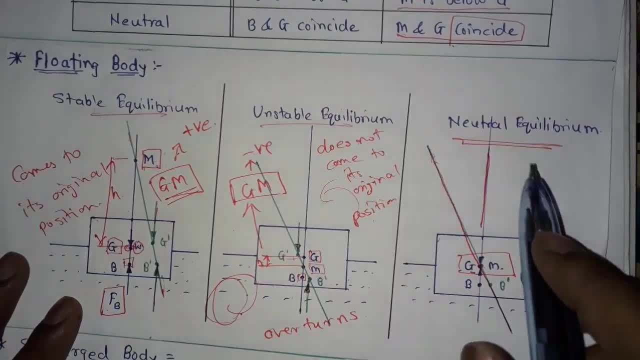 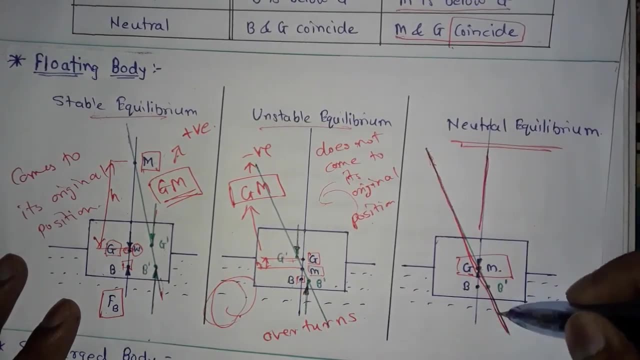 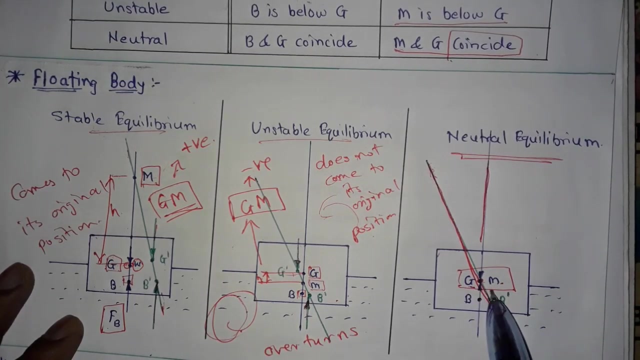 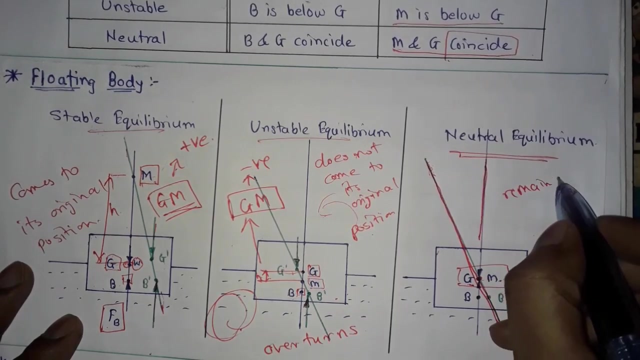 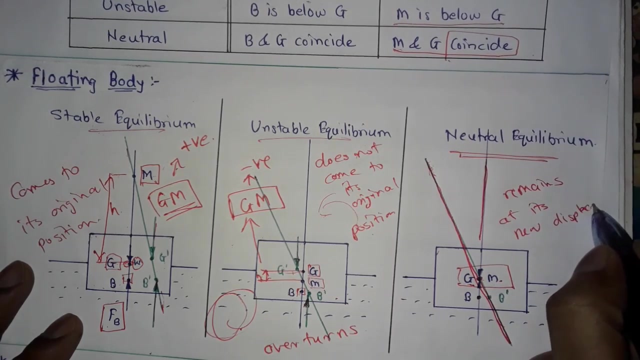 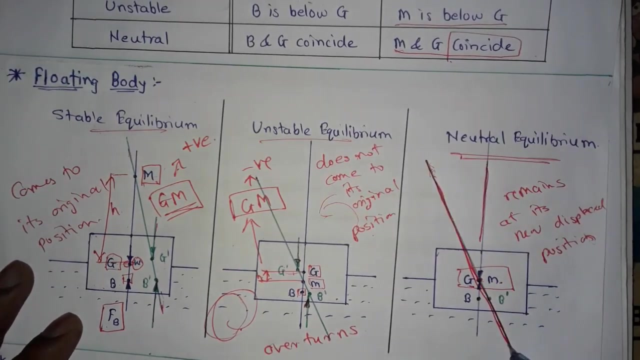 displaced axis in neutral equilibrium condition. friends, body remains in this new position in neutral equilibrium. as the G and M acts at the same point, body remains at its new displaced position, that is, in this case, this is new displaced position, friends. next is friends: submerged body for stable. 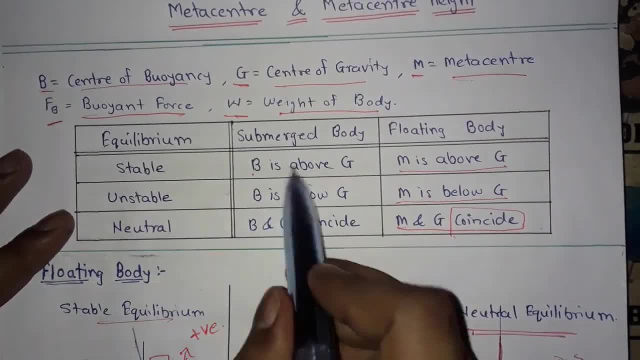 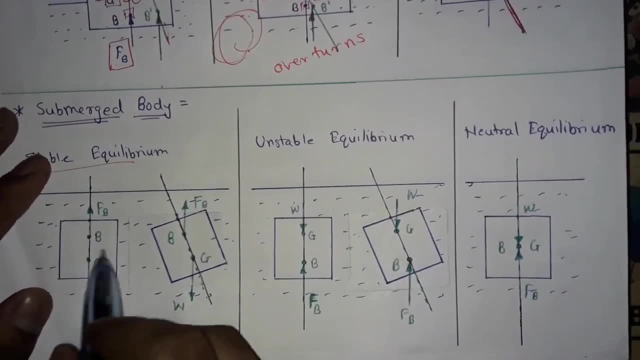 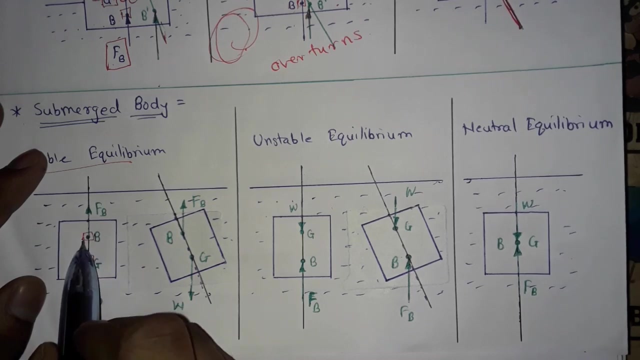 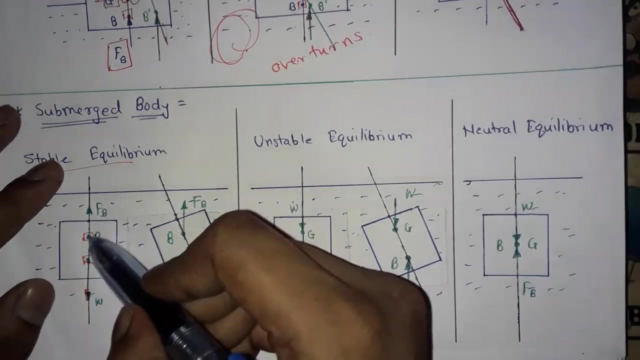 equilibrium, friends, in case of submerged body, B is above G, that is, by by. the center of buoyancy is above G. here, friends, this is fully submerged body in the liquid. this is center of gravity and this is the center of buoyancy. here also, friends, weight of the body acts downward at G and buoyant force acts above at the. 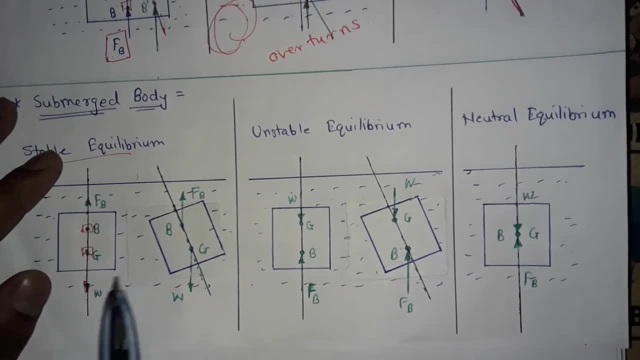 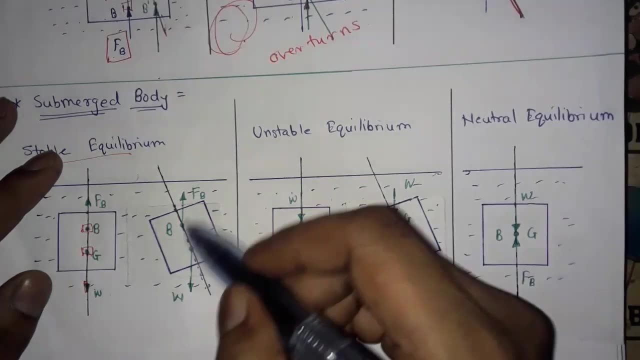 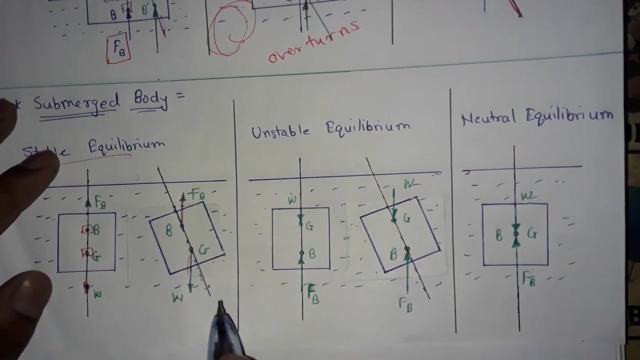 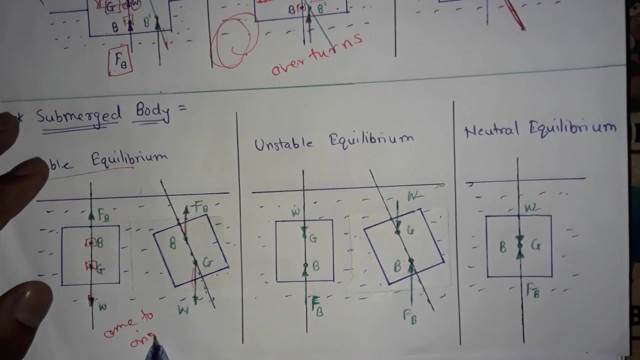 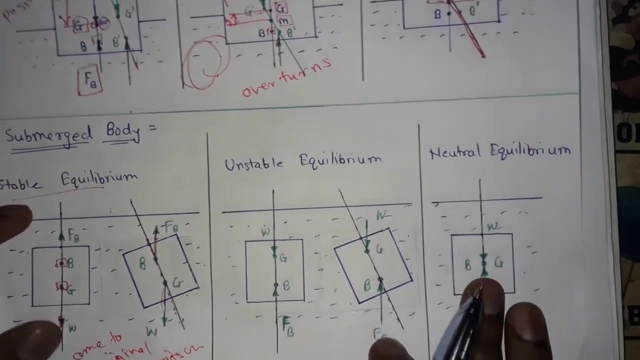 center of buoyancy, in this case, friends. if we displace body from its original position like this, like this, friends, there is all. there also couple forms like this, and and due to this couple, friends, this body come to its original position, come to original position. position in this case, friends, and next is friend, unstable equilibrium. 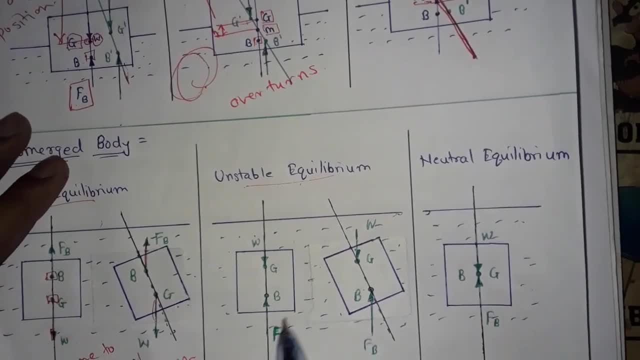 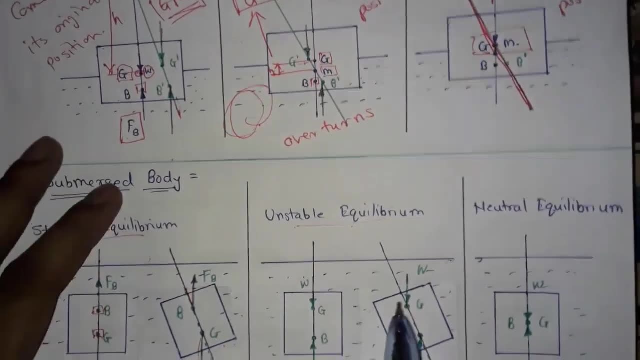 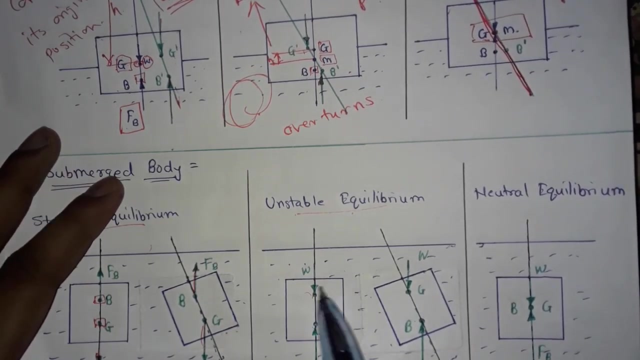 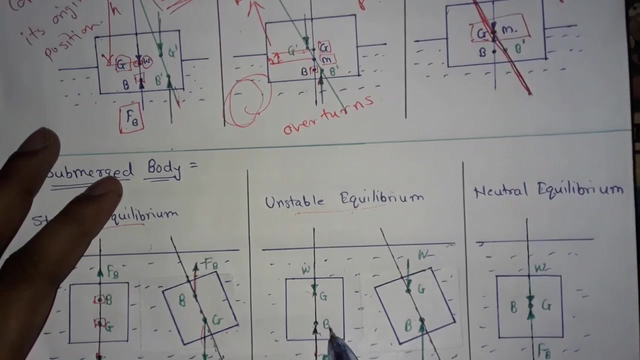 in this case friends, friends, in this case friends. here, friends. I will show it here two times here. G is like this about this 寸 after this: now, this is boundary of pull wind position. it gets affected by gravity. friends, here we take a close look. here I will expand my 그래on stop. weight of the.